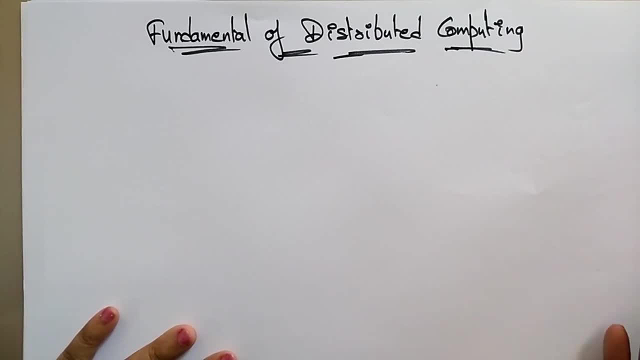 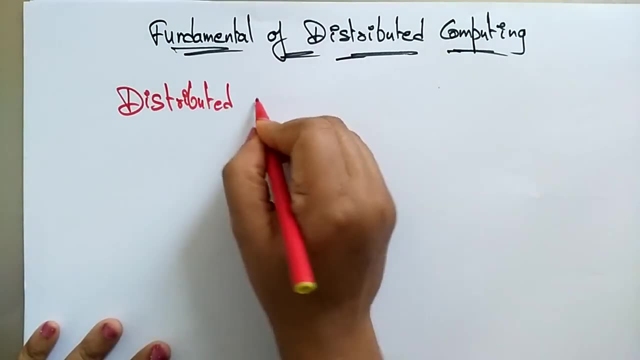 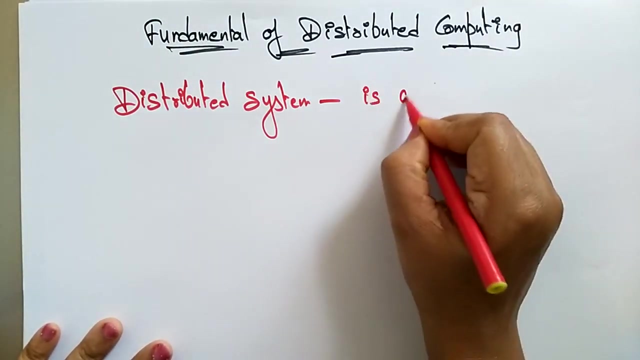 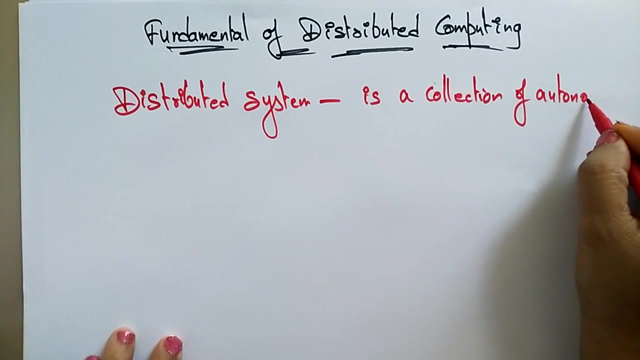 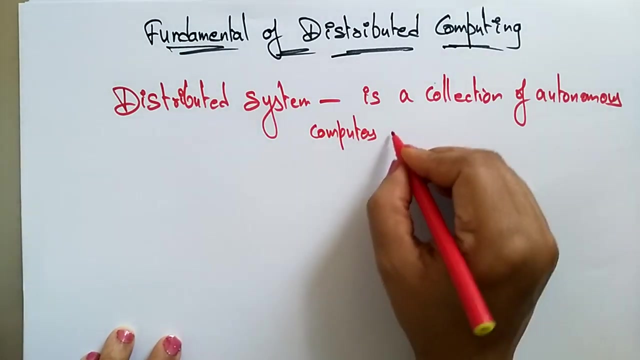 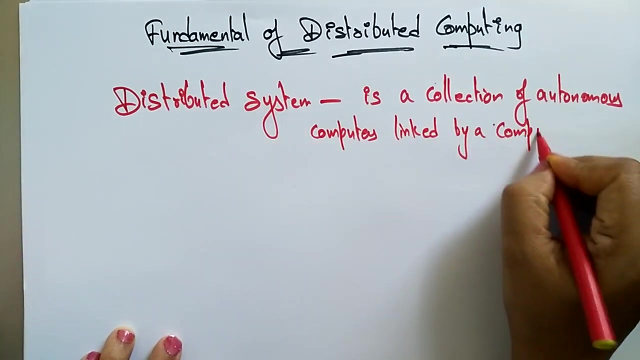 so, first of all, what is this? distributed computing or a distributed system? a distributed system: okay, so a distributed system is a collection of autonomous computer. is a collection of autonomous computers linked by a computer. network means these autonomous computers are linked by a computer, a network, and all these equipped 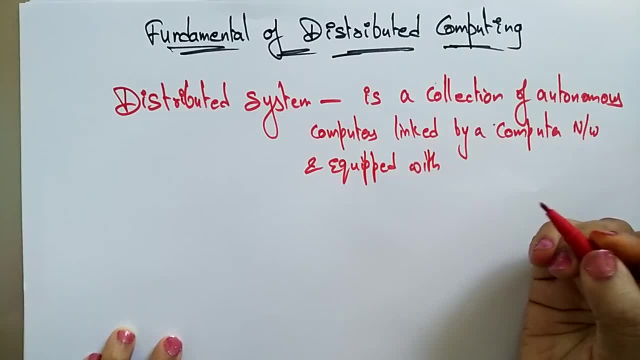 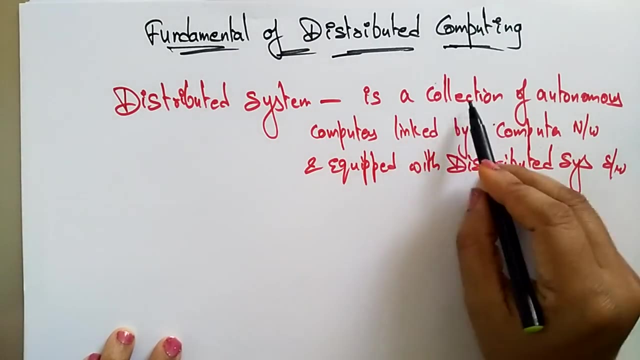 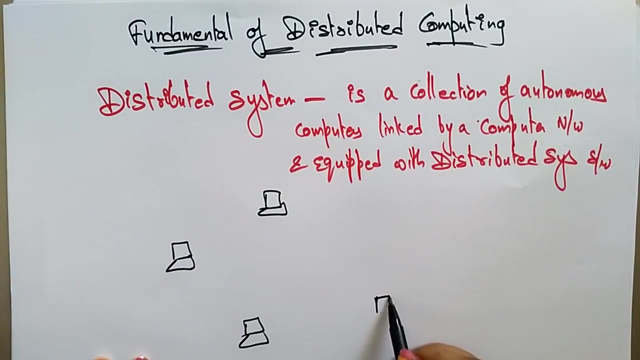 equipped with distributed system software. distributed system software, that is a middleware, okay, so let me explain you with the diagram. a distributed system is nothing, but i'm saying it is a collection of autonomous computers, means the different computers are present. it's a collection of autonomous computers. autonomous computers, okay, or autonomous computers linked by a computer network. 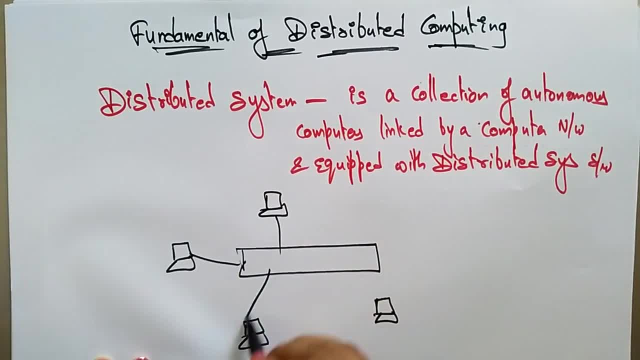 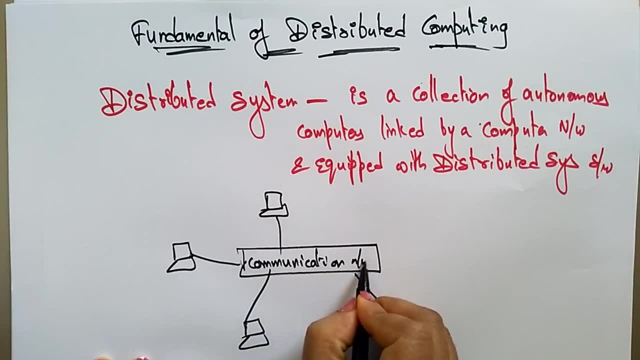 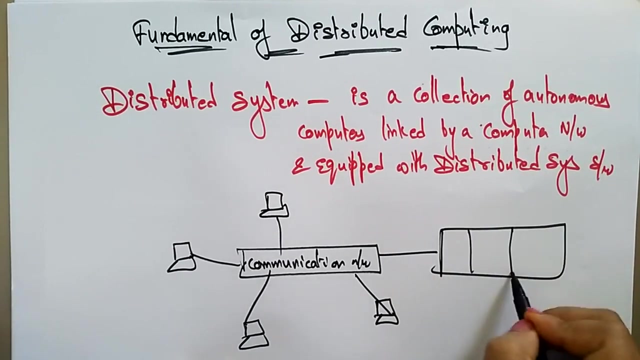 means this: everything or linked by a computer network, so which you call it as a communication network. a communication network and all these are equipped with a distributed system software means each and every system is having their own systems and all these are equipped with a distributed system software. so this is a distributed system software, so present a different. 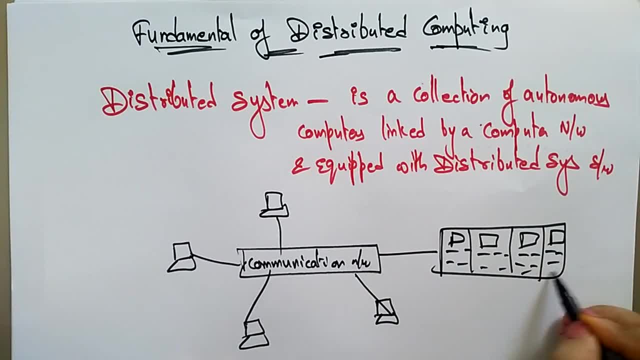 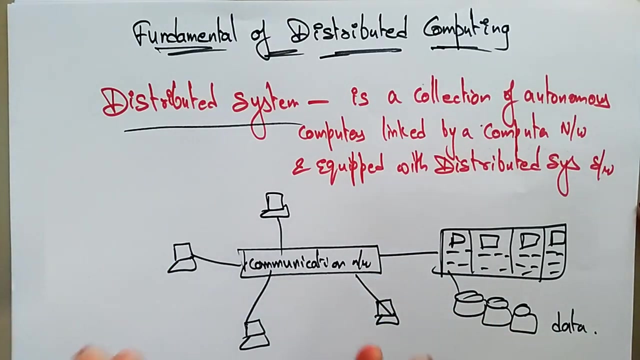 servers. okay, all are equipped with a database. so this is a data. so this about the distributed system. a distributed system it's just a collection of autonomous computer. so different computers are means the independent computers are communicated with the help of the communication network. means all are linked by a computer network and equipped with a distributed system. 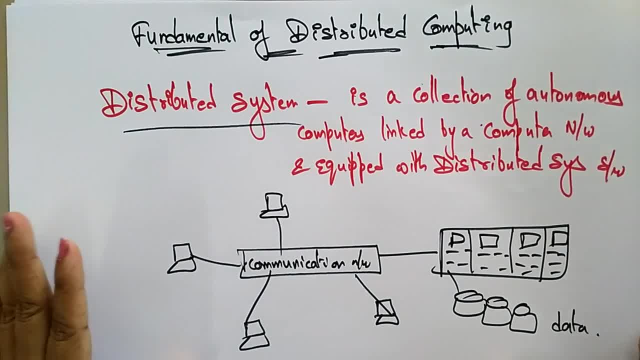 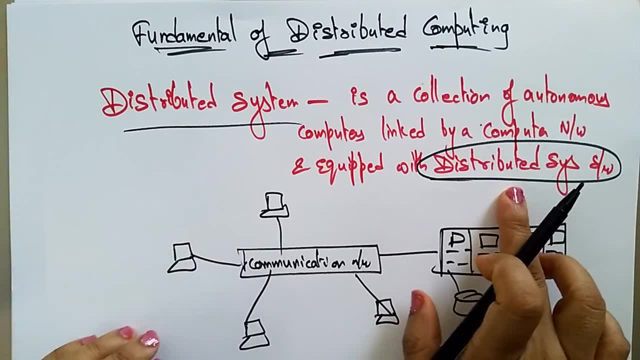 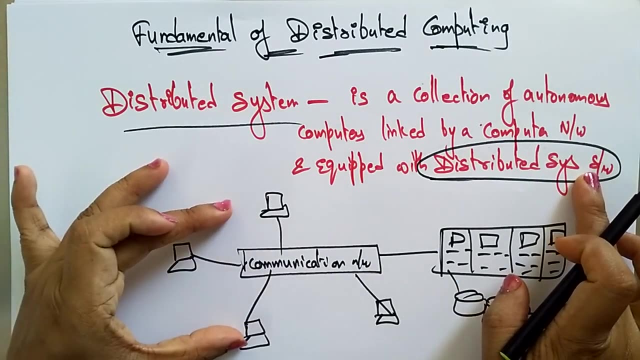 software. so that is the exact definition of the distributed systems. so actually, these software, so whatever the software that I said, the distributed system software, this software enables the computer. what exactly the role of this distributed software? I said these computers are linked by a communication network. so why they are linked with this computer network? 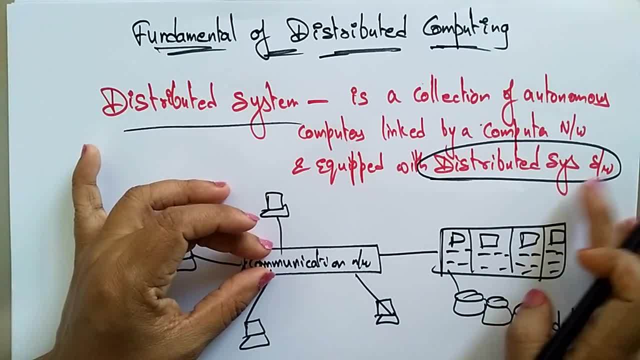 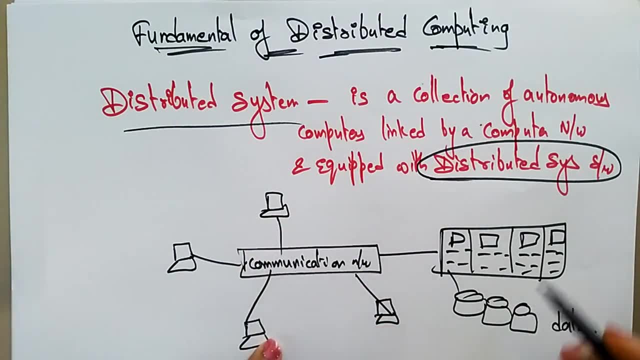 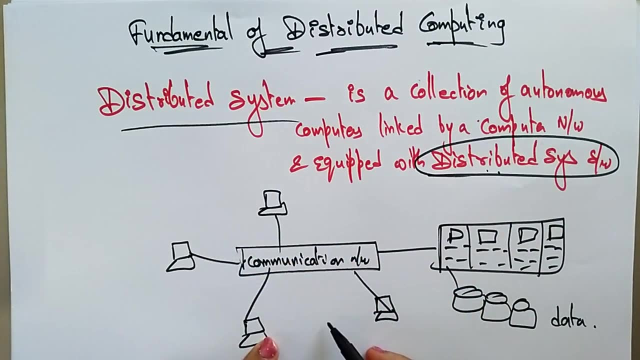 because of equipped with distributed system software. so this enables all these computers coordinate their activities. so the main use of this distributed system software is to coordinate different computers activities and to share the resources of the system: hardware, software and the data. let me write that point so that you will remember that. so this distributed system software. 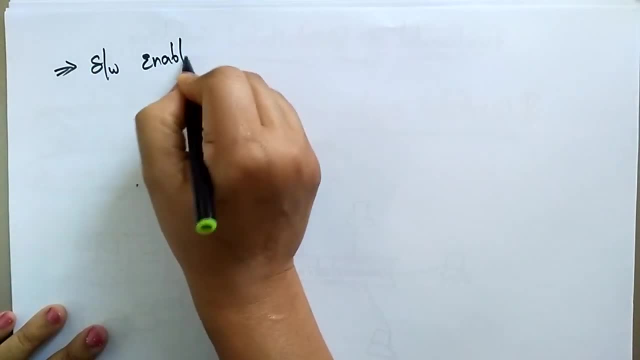 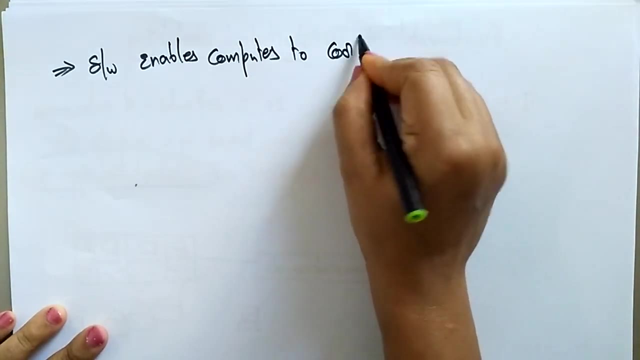 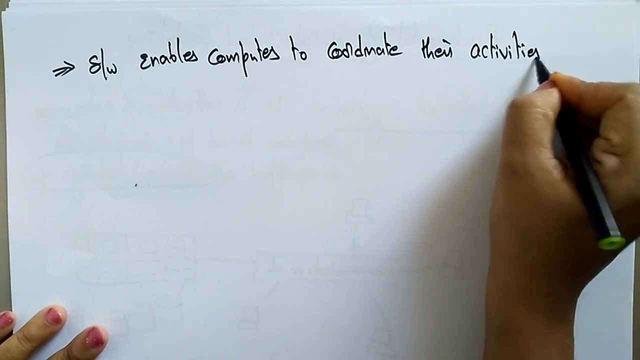 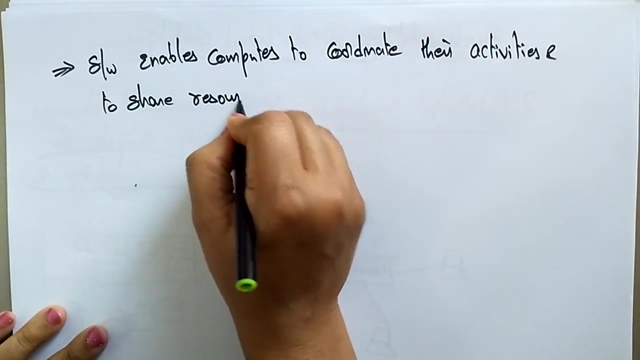 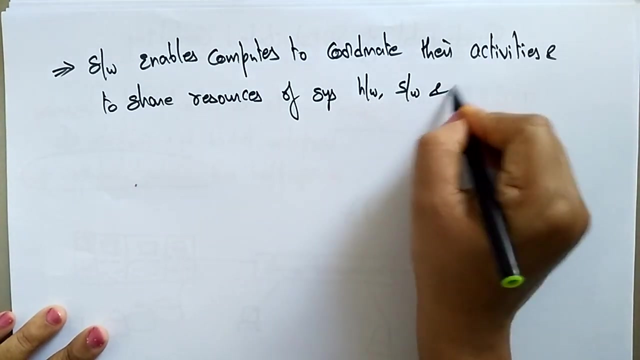 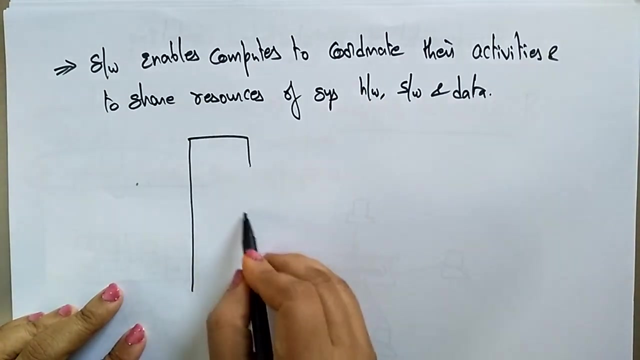 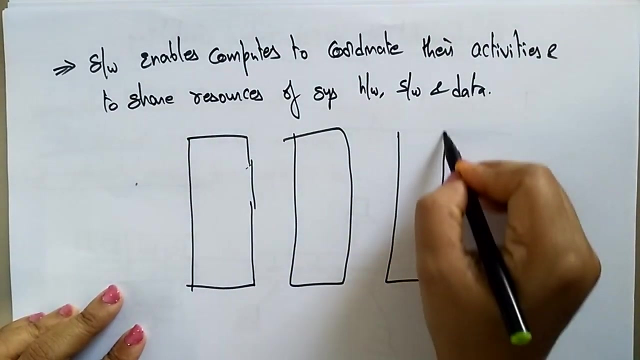 enables computers to coordinate their activities, a mutual exhibition, coordinate their activities and to share the resources, whatever the resources that each system means is having, like hardware, software and even the data also. okay, let me show you. let me take a: there's a machine a machine B. let me take it autonomous. 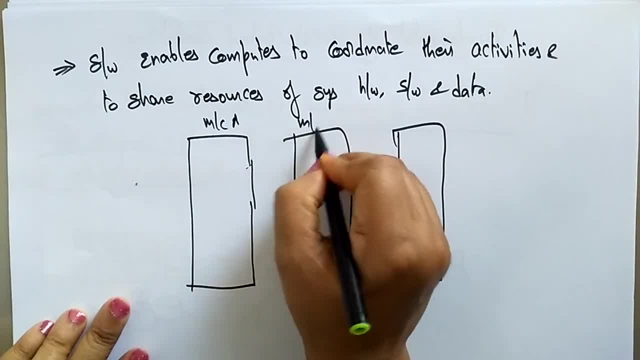 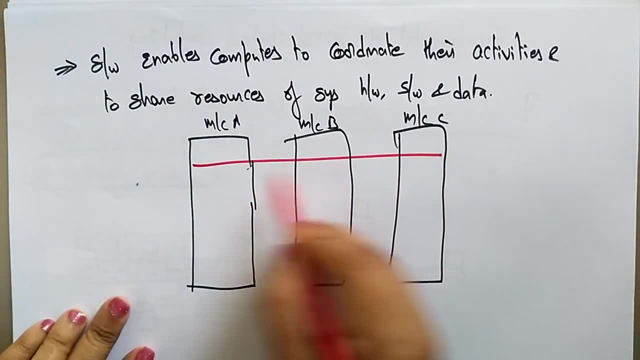 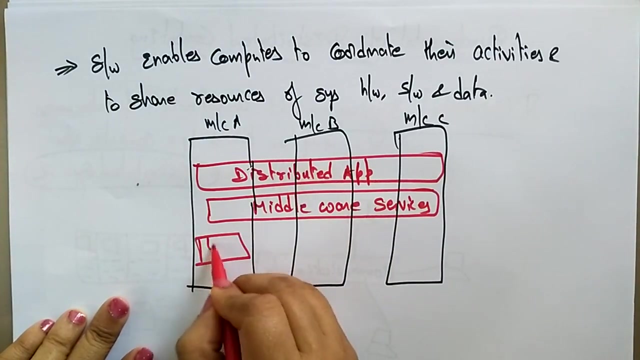 computers at three different computers: machine a, machine B and machine C. so these may, all machines are having the distributed applications, a common distributed applications, and all these machines have a common middleware services, middleware services, and each machine is having their own local operating system, their own operating system. 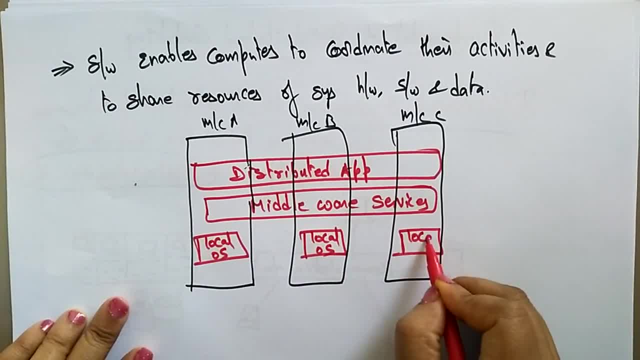 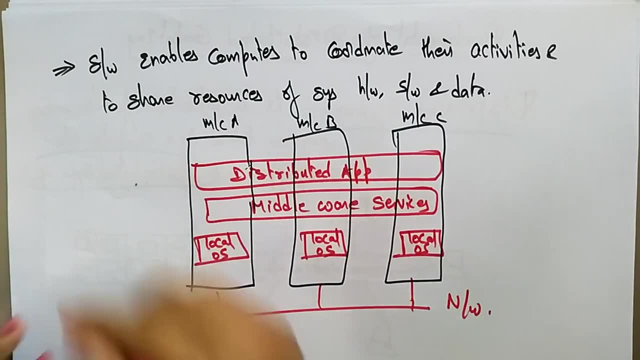 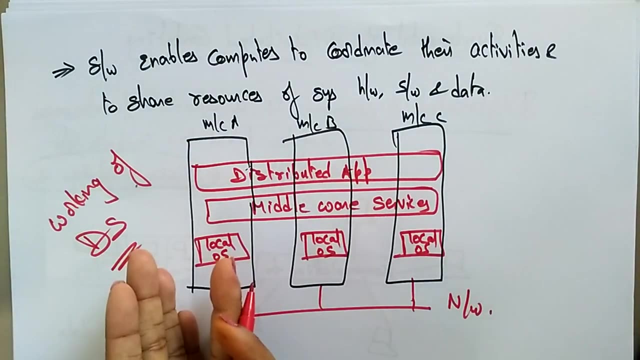 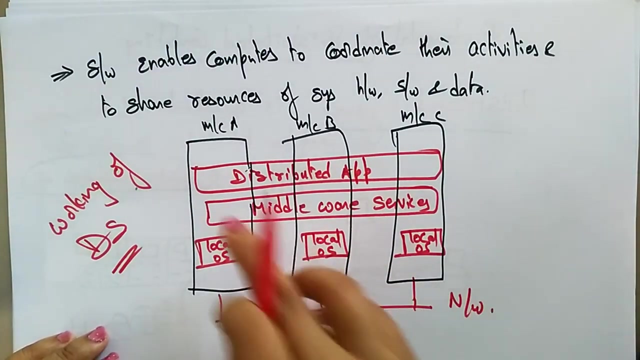 you, you and all these systems are connected with it network, they are connected in a network. so this is exactly the working of the distributed system, working go distributed system. so here you are, taking the independent autonomous computers. it's a collection of autonomous computers. all are linked by computer network and equipped, but with a. 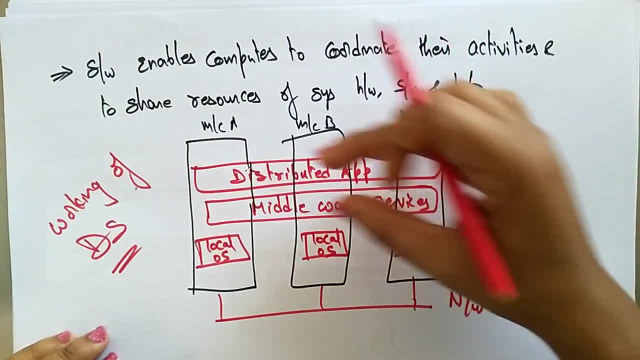 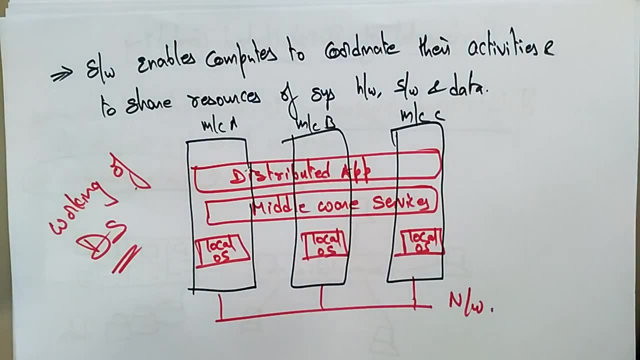 distributed system software. so these are all equip directly each machine is excepted the distributed system software, that is, the distributed applications and the middleware services. so this is exactly what a distributed computing or distributed systems are. so whenever they are asked about what is a distributed systems, try to explain the definitions with the diagram.